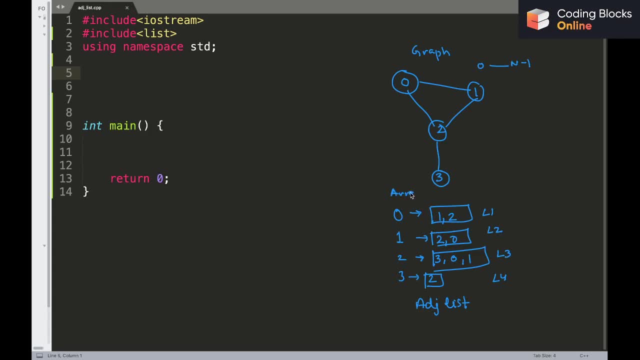 And accordingly, I can create an array of lists. Okay, so I can create an array of lists of size v. That means I have v number of arrays, And each array- the zeroth array- will store what all neighbors are there for the zeroth node. First array- will store what all neighbors 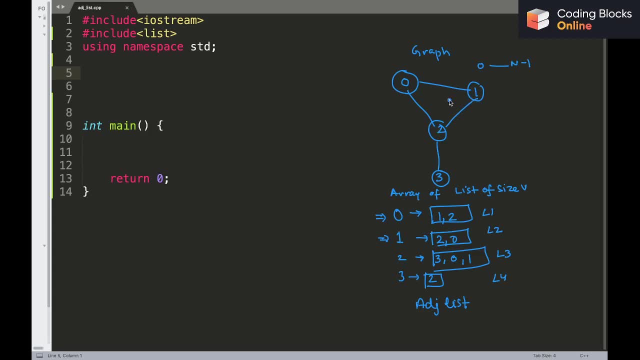 the first node has. So first node has only two neighbors, that is, two and zero. So they will go in the list of the first array. Okay, so what we will do is we can start by writing some code. So let me define a class. 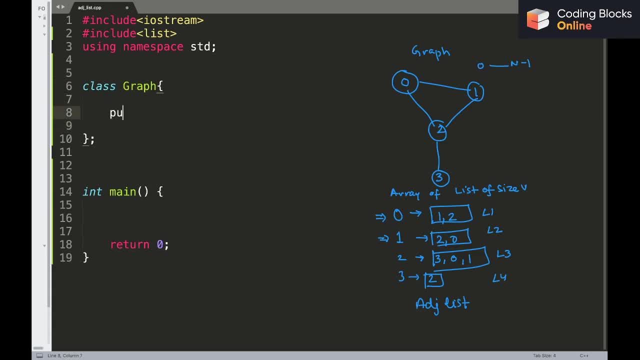 called graph. that will represent my data structure and public. I can make a graph constructor Where I can accept, okay, how many nodes this graph has. So I can define a data member v, and I can say, okay, this arrow v equals to v. So this will basically said: okay, we have. 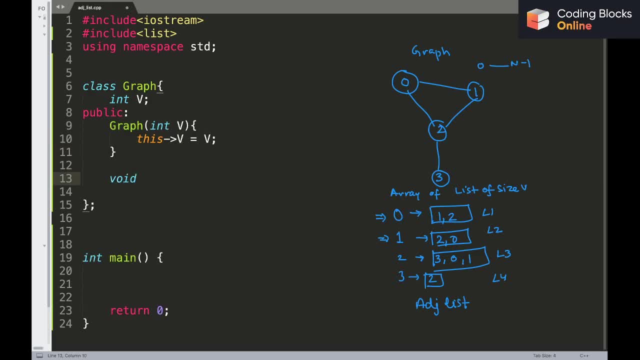 vertices in the graph and maybe we can create a function called add edge. okay, and since there is an edge between two nodes and each of those are integers, i can say, okay, int x and int y. so what i can do is, if there is an edge from x to y- and i'm assuming it's a bi-directional edge- 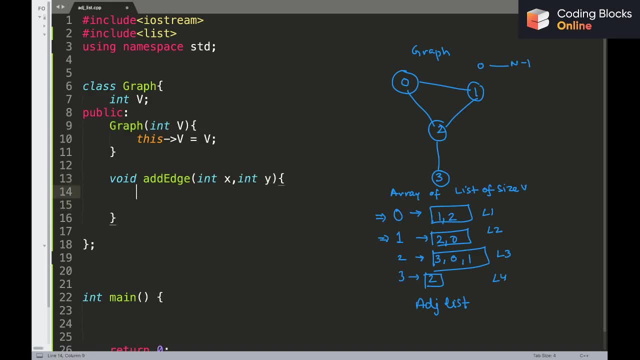 so what i can do is i can say, okay, i need to make a array of lists, okay. so if you need to make a single list, then this can be written like this list of integers as l okay. but if you need to make an array of lists, so we can say, okay, whatever is the size v, we can use it, but this v. 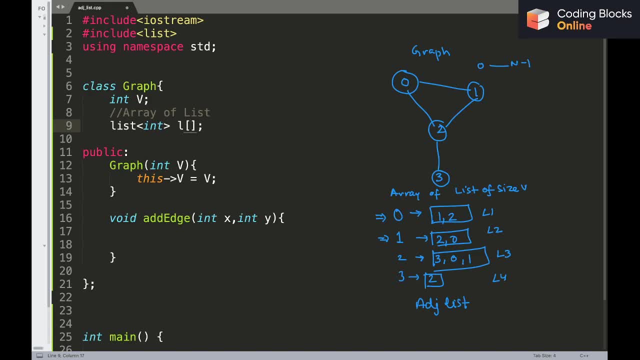 is not known to us during compile time, but it will be known to us during compile time so we can use it. but this v is not known to us during compile time, so we can use it. but this v is not known to us during compile time, so what we can do. 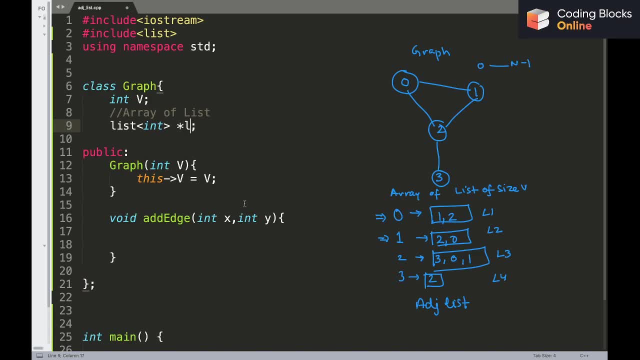 is, we can keep a pointer to an array of lists and this we can initialize once we know the number of vertices. so i can say a list int star l, this is equal to new list int of v. so that means l is a pointer to an array in which each element of the array is a list. 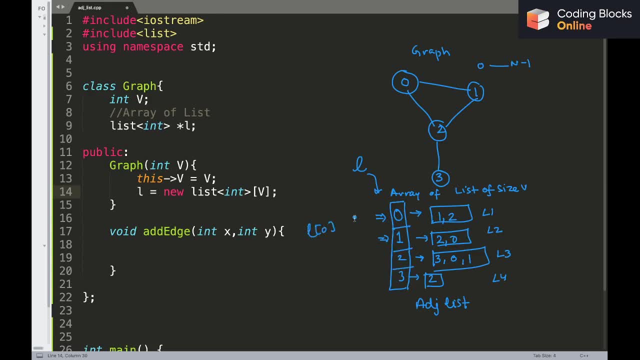 okay, so if i talk about l of zero, then it means this whole list. if i talk about l of one, it means this whole list. so l is a pointer and it's a pointer to an array of lists. okay, so if you just write it like this, it's equal to new list. so that means you're. 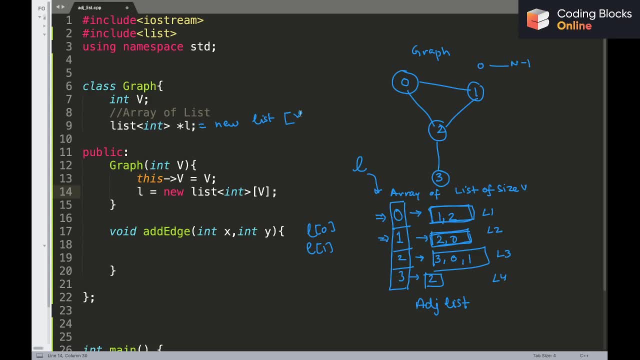 creating a list dynamically and if you say, okay, no, i want, instead of one lists, i want v lists. so this is actually an array of v linked lists. okay, so this is. you can see. this is the first linked list, second linked list, third linked list and the fourth linked list. this is the first linked list. 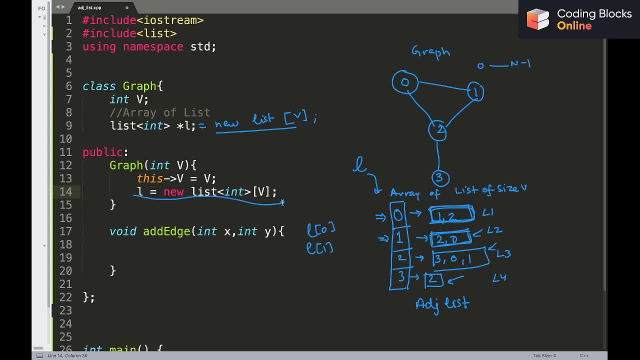 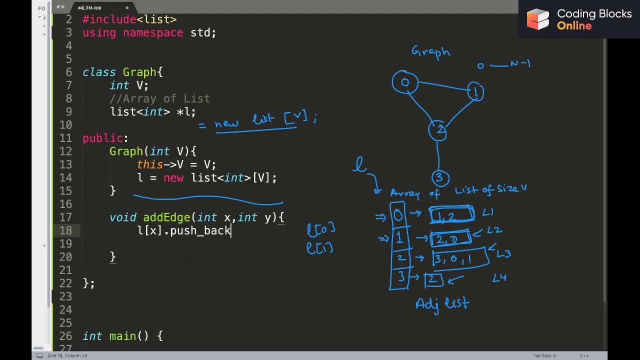 this is what we can undo here. so i have initialized this inside the constructor and if you need to add an edge, then it's also going to be simple. you can say: uh, if there is an edge between x and y, you can say l of x, dot push back y, and you can say l of y, dot push back x, and that's it. so that will simplify. 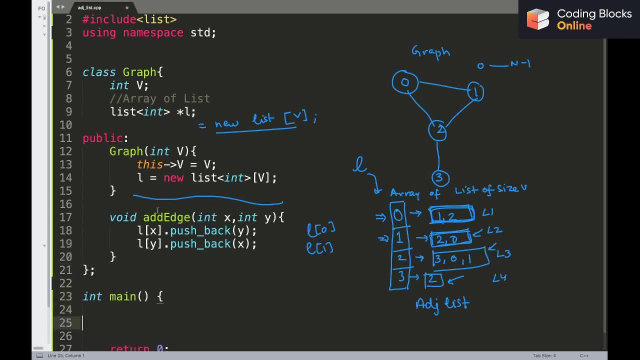 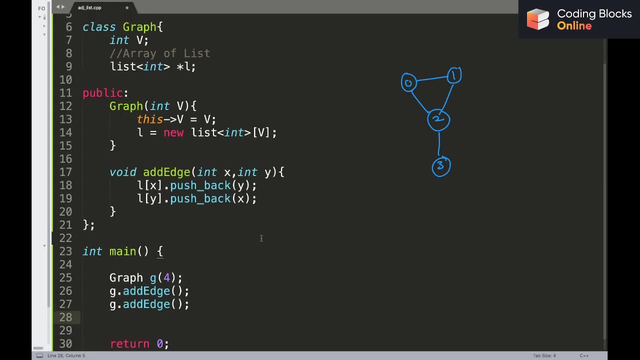 the work for you and you are done, okay, okay. so what we can do next is: uh, we can say, uh, let's create a graph with four vertices, so i call the constructor, and if i want to add edges, so i can call this function: g dot, add edge. and here i 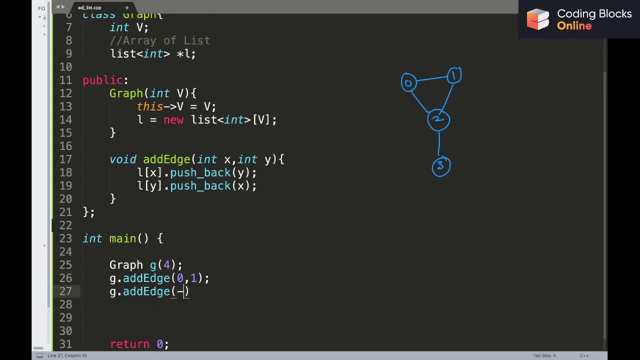 can say: add an edge between zero to one, add an edge between zero to two, and also add an edge between two to three. okay so, since i have uh four edges, so one more edge that i need to add is between one to two. okay, so, this will add all the four edges and these are uh bi-directional edges. okay, so here what we have done. 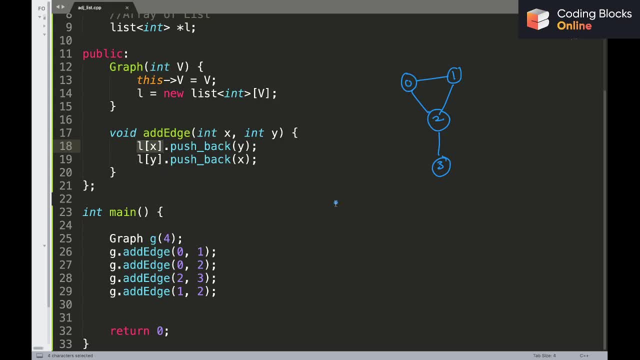 is. list has a function called pushback. so i say l of, let's say l of zero dot, push back two, so that basically does what it does. it does is we have a linked list, zero- and in that i push back an element two. so if i say zero is connected with one, i say okay, zero is. 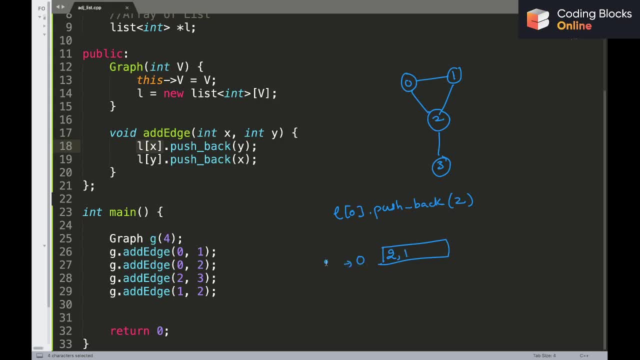 connected with one. then l of zero dot push back one. so in the zeroth link list i push two elements, two and one. so that means zero is connected with these two particular elements. so now let's also try to ah print it. so if you want to write a small function that will actually print the adjacency, 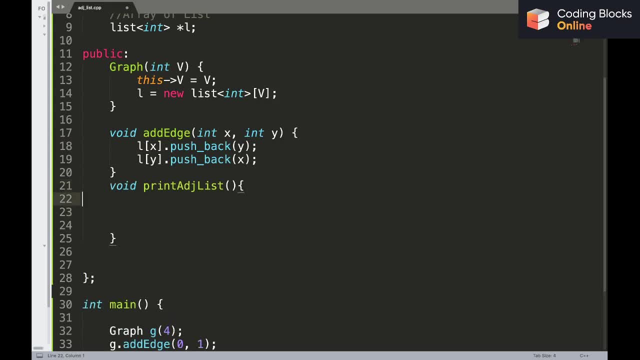 list. so in that you you can iterate over this particular us four edges and you can see under this list, one connection line is just what is being loaded now but frequentlyStarting toast which is the elements. okay, so you can say let's try to iterate over all the vertices. so 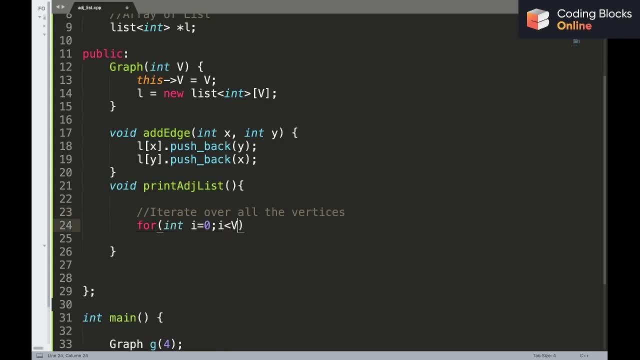 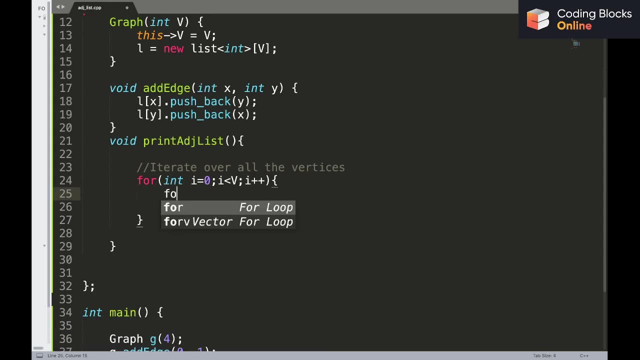 you know we have V, V vertices. for int I equals to 0, I less than V, I plus plus, and for every vertex you need to iterate over that particular linked list. so I can say: for int X, that is there in L of I, okay, so either you can use this kind. 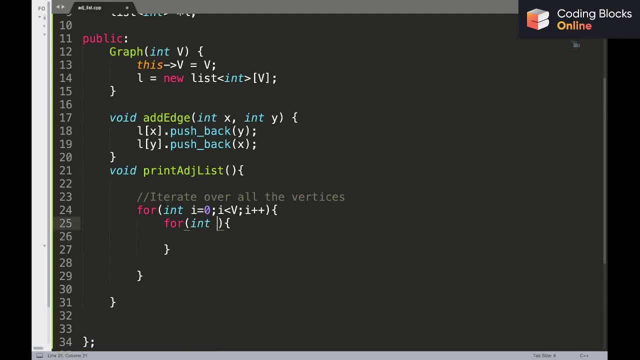 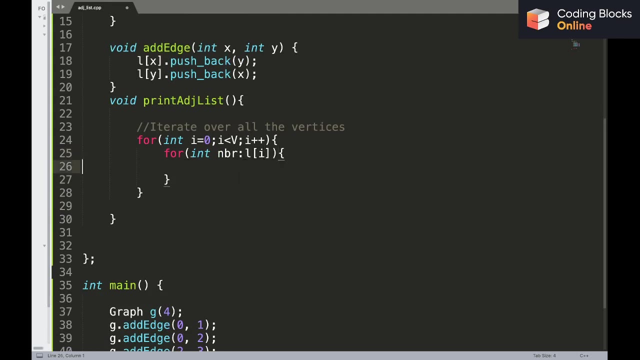 of a loop or you can use an iterator so you can say auto neighbor or int neighbor. let me write it like this: only so: int neighbor, that is there in L of I cout neighbor. okay, so this is one way, and here we can just print: we are on this. 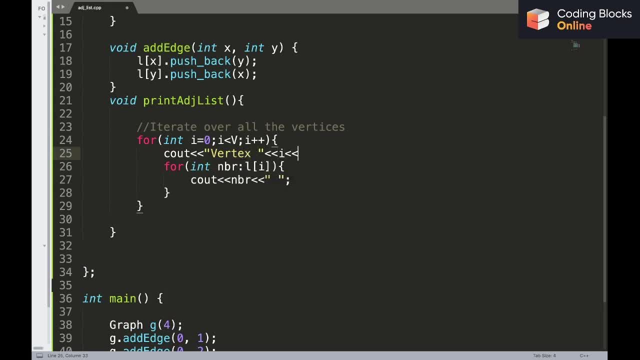 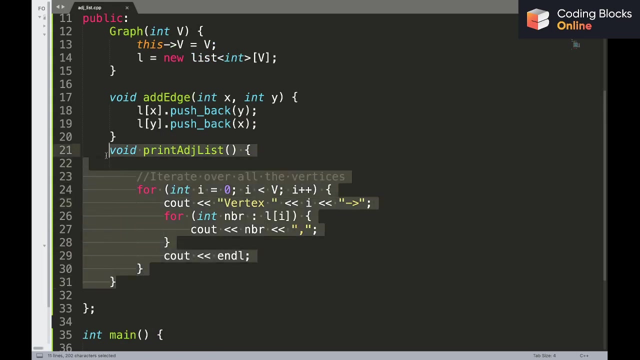 particular vertex, and that vertex is I, and followed by the neighbors of that particular vertex, and after every vertex I just print a end layer, and after every vertex I just print a end layer. okay, so we have written the code to print all the adjacency lists. so what we? 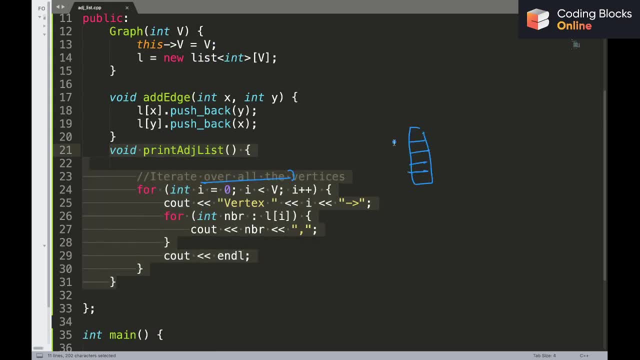 do here. we go from the 0th linked list till the Vth linked list and for every linked list we say: okay, we keep a variable neighbor that iterates over the Ieth linked list. so Ieth linked list contains all the neighbors of the node I. 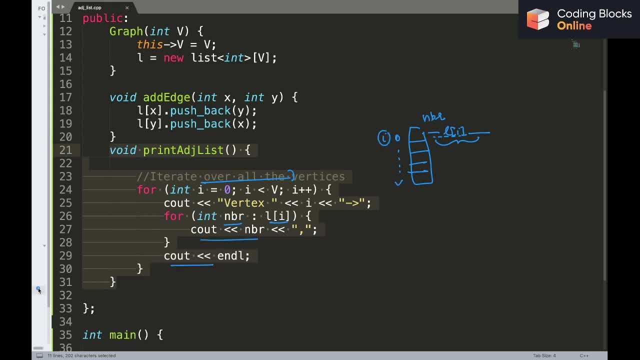 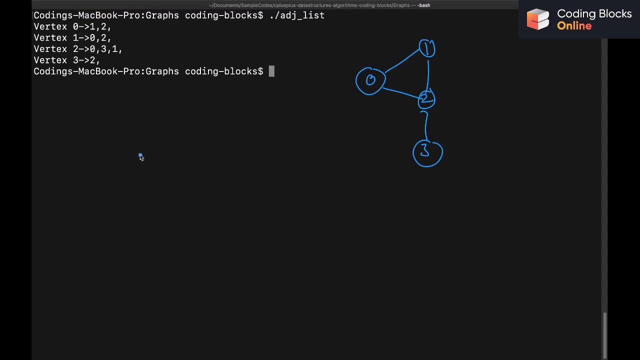 and that's how we get all the neighbors, and after every neighbor we press a handle here. so let's try it out, let's try to run this code. okay, so let's see the output. now you can see this is the output of the print function and you can see 0 is connected with 1 and 2.